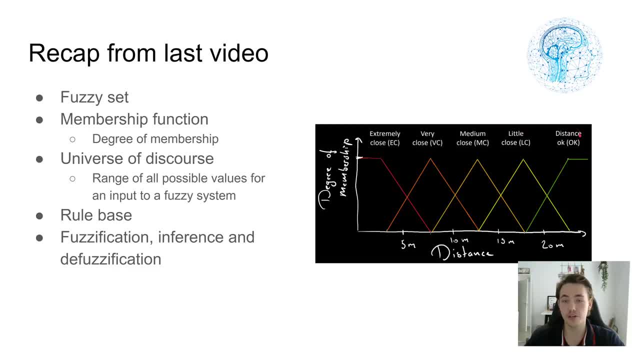 extremely close, very close, medium close, little close, or, if the distance is okay, so it's the distance to the, to the car in front of us. and then we set up our fuzzy set and our rules like: so We divided it up, like this. and then we set up our rules like: so We divided it. 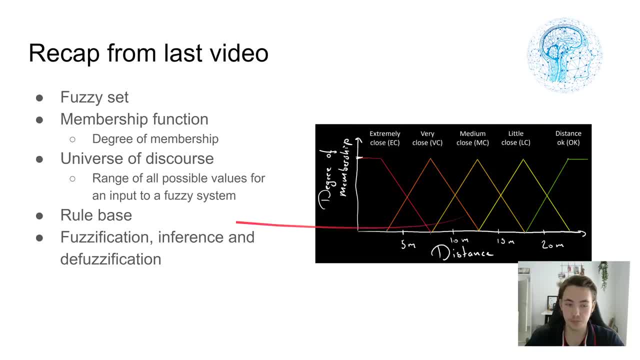 into, like smaller chunks that we can then like have a membership function here which, like, tells us like what degree of membership each like, like each set, has. So in this case here we can see: like, um, it's, it's not, it's not either like boolean, um, it's not boolean logic, where we can only have like. 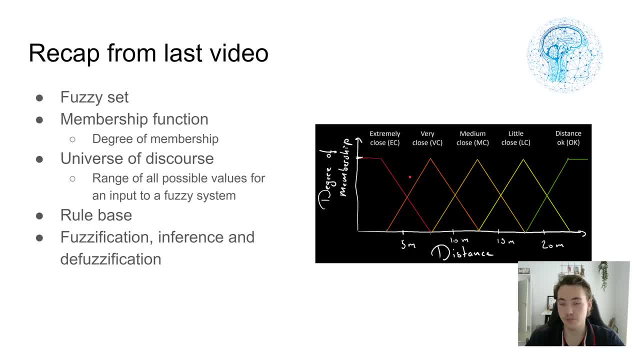 zero and one. but here we can have like some degree of membership for, uh, for our fuzzy sets. So in this case here, like we can see, like up here we have one, but then like it gets lower, lower, lower, because like we get like um farther away from the, from the car in front of us, but like not like a. 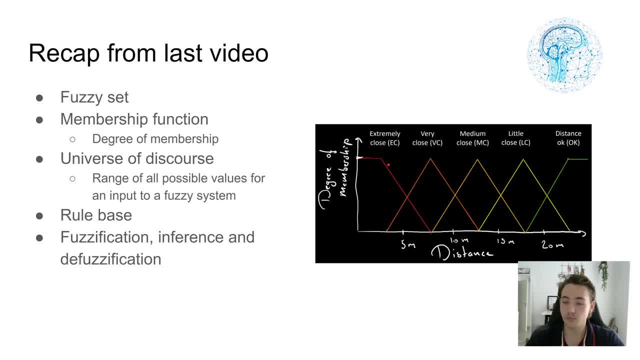 zero, and so we don't have like this crisp, uh, crisp, um, crisp, translation from one state to another state or from one set to another set, So it just gets like um less and less extremely close, and then it gets more, more, very close here, as we can see here, and this is like just like how our 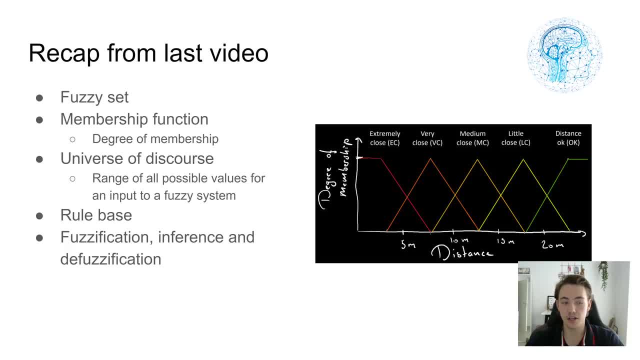 membership function. in this case here is, is defined, And then we have, like, our universe, of course, which is down here on the x-axis and in our example from last video where we had the distance here to the car in front of us. So it's the range of all possible values for an input to a fuzzing. 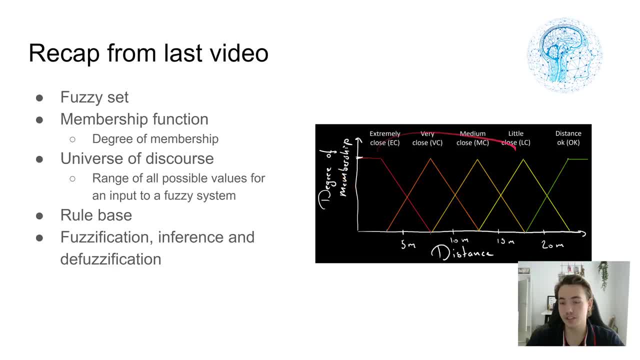 system. So in this case here, like we have these kind of inputs here where, uh, the cars can be in different kind of the different kind of states for for the distance, and then, um, every like, every like distance can have some degree of membership in in our fuzzes sets, And then from all of this we just 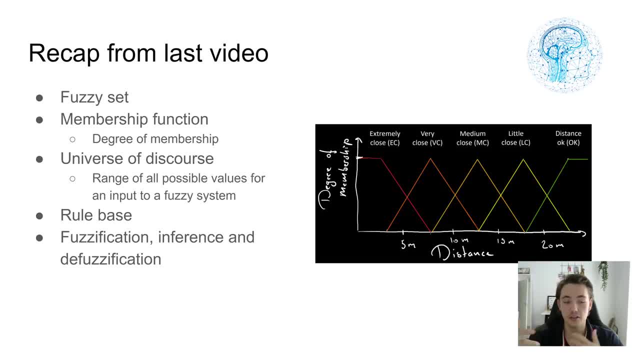 then we can use um, our rule base for um our controller in our controller and use this. these are the falsification inference and these are the defazification that we just went over in the last video And these are like the topics that we're going over in more in depth in this video, and I'm 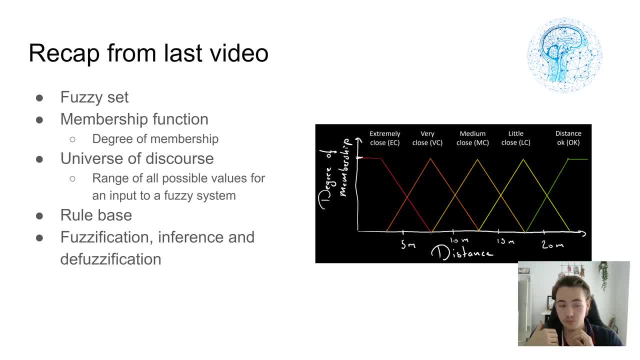 going to show you, like, how we can uh, fuzzicate, um, fuzzicate our crisp value and then inference with our rule base And then in the end, like you do these defazification to get, um, a fuzzy logic value to a boolean value and a crisp set again that we can apply to uh, to our system. 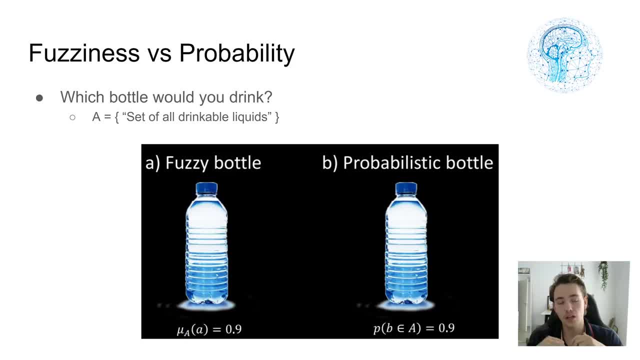 So first of all, I just want to like, uh, give you an overview, or like what, what is fuzzing it, uh, compared to probability? because a lot of people they think that that they're like kind of the same, but but they're really not, because if you, if you see the sample down here in the button button, we have two. 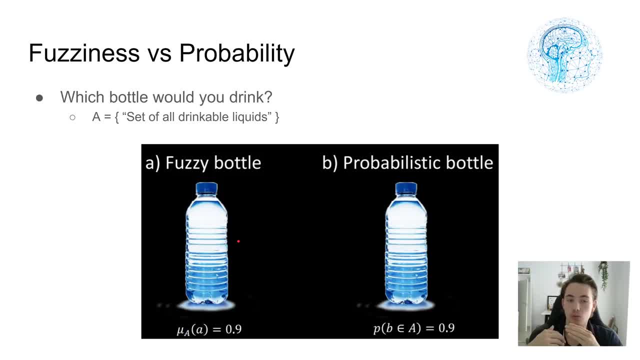 bottles and that the question is then: like which bottle would you like to drink? and a is like, the set, is our, is our fuzz set here, which, which is a set of all drinkable liquids. So in the example here to your left, we have a fussy bottle, which means that, like um, our degree of membership is 0.9 would mean like it's. 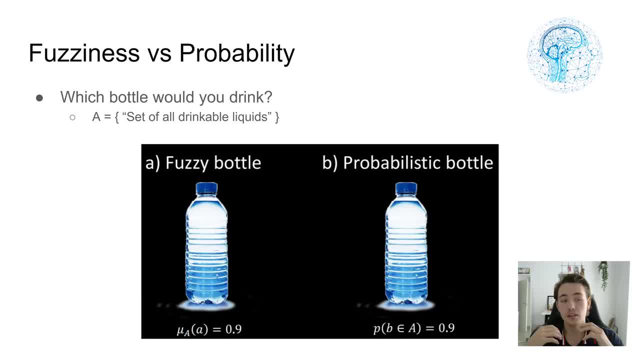 not like it's. it's 90 percent uh drinkable, but like the like the liquid inside of the bottle is like nine percent um, uh, like the probability, like, not not the probability, but like it. it should be like uh eight and the nine percent of the of the of the liquid inside of the bottle. 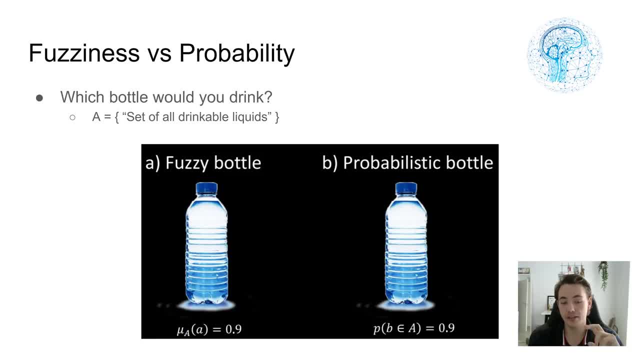 is is drinkable. so like, let's say, like it's 90 water and then, uh, 10 something else, so it's a pretty drinkable. um, it's pretty drinkable water if the fuzz bottle has like a member degree of nine. point a lot of 0.9 uh in in case of the fuzz bottle here, and if we're talking about like a 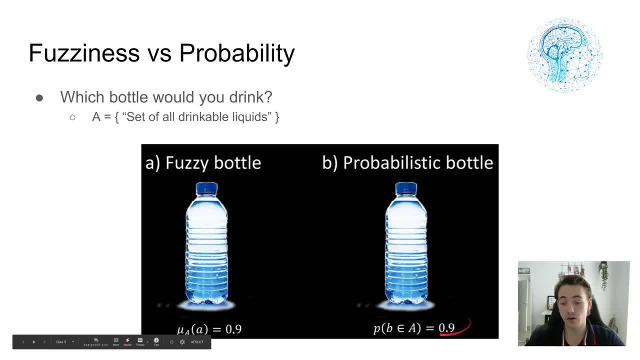 probability and we have like the bottle here to write and we have a probability of of 0.9, then we have a 90 percent change that this is like drinkable and we still have like a 10 chance that it's not drinkable or if it's acid or something else like that where over here. 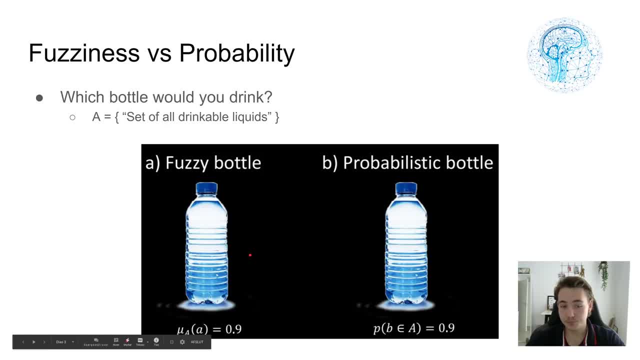 like. it's just like nine percent of the volume inside of the of the bottle is like it's drinkable and then the other 10 percent uh could be like uh less drinkable than like, for example, water. so it could be like coke here and then like over here we have like we wouldn't drink a bottle of of uh a. 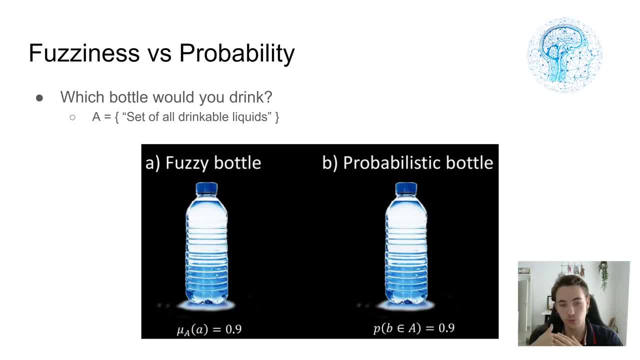 bottle if we only had like nine percent chance that that it was drinkable or like 10 that it was acid. so like it's, it's very- it's very useful to know like difference between like fuzz bottles and probably based uh, probability, uh, because they're two different kind of things and people sometimes 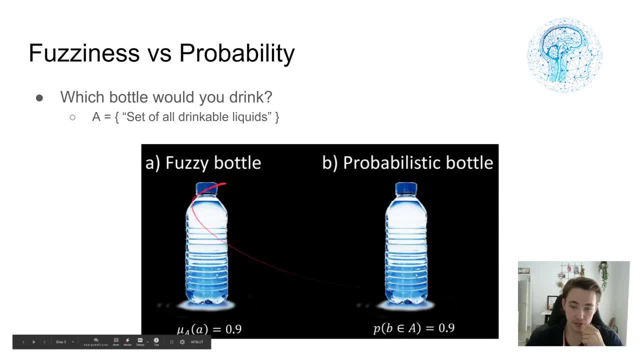 they um, um, they think they're the same and like think about it in the same way, but they're really not. so when we're talking about like fuzziness, we need to to like think about it in in the way of like, how how much degree of membership, um, does this value here containing our thoughts? 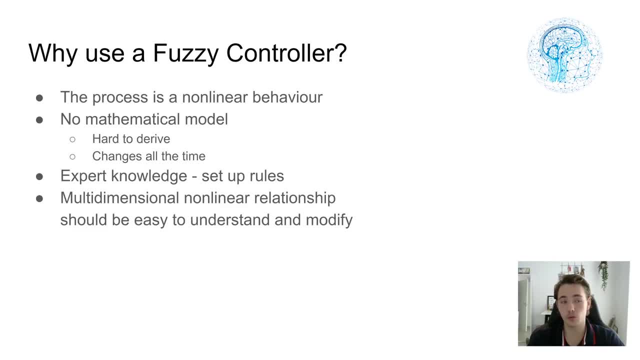 so why? why are we using fuzz controllers and what can they be used for? so we're often using fuzz controllers when the process is is a non-linear behavior, because then it's hard to like set up a um a controller like an, a classical uh controller, because, um, when we have this fuzz controller here, 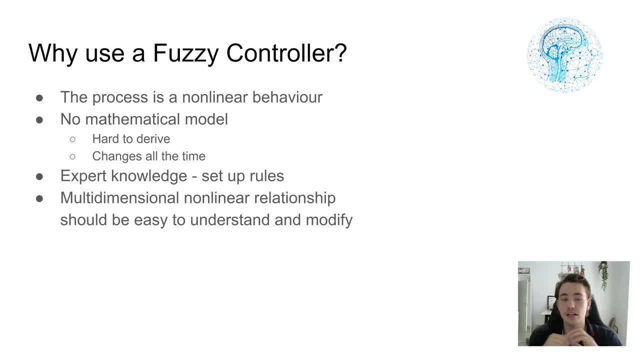 we just like we can just set up our rule, set our rule base and set up our fuzzy sets and then have some some kind of like um membership, uh, um degree function that we can determine ourselves, and then we can just use our fuzz controller in that way. and also, if you have no mathematical model, because it cannot be like hard to derive- 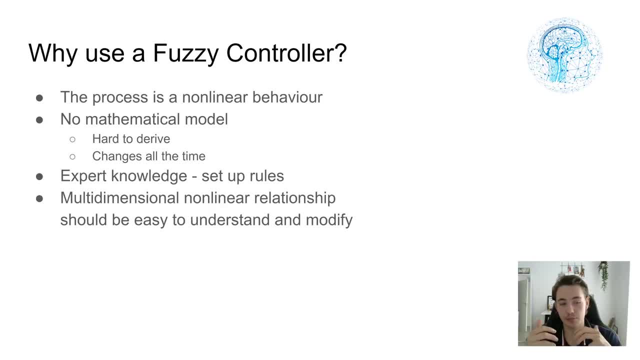 or it changes all the time and often in practical examples or applications, like it's just really hard to to come up with a mathematical model and sometimes they're like really complex so like there will be a lot of different kind of like noise to that model. that that is not like taken. 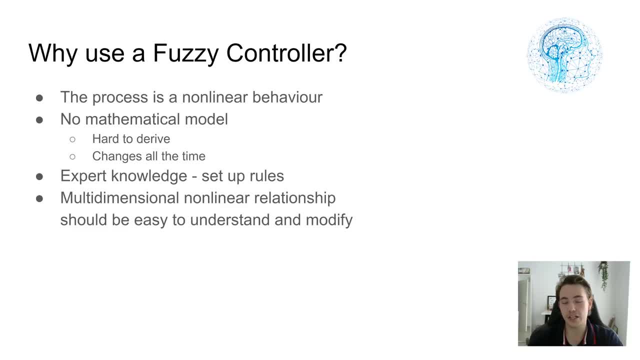 care of or or taken into account. so a fuzzy controller you can actually like be better than to to derive a mathematical model and try to like implement some of the controller that needs a mathematical model and also, if you have like, for example, an expert knowledge, if you want to like um implement a. 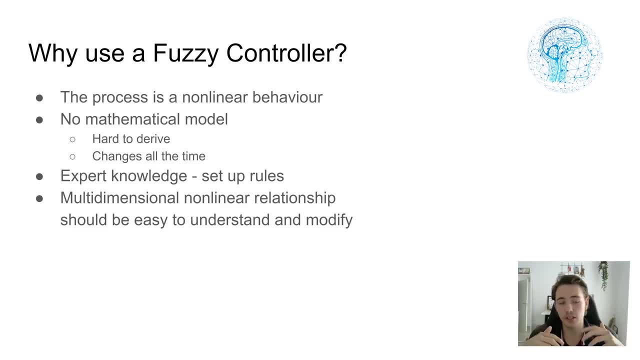 controller for someone and they're, they just come here like, for example, in the car example, like I just- uh, if I just talked with to like a guard, that guy that wants some kind of like autopilot, they can. they can like change the speed compared to like how, how far it is. 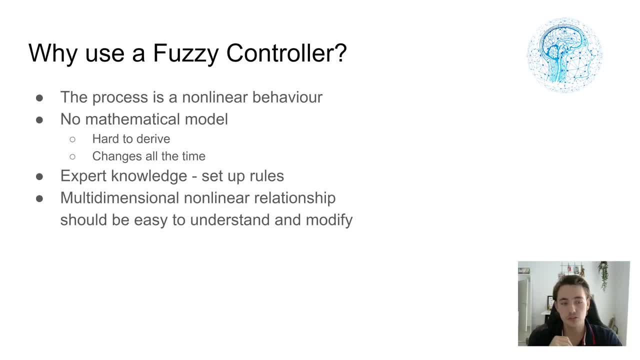 like behind or another car in front of it. so then the expert could just say to me like oh, if the car is like um far away, then drive at this speed. or like um, and if it's like close to it, and drive at this beat. so like it's easier to set up rules and for a fuzzy control and then we can just use. 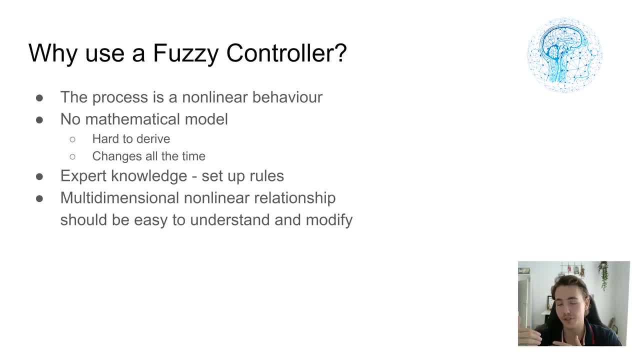 those rules that is set up by the expert that we want to implement the controller for, and then we just set up our rules and apply our fuzz controller to that. and also, if we have like a multi-dimensional, non-linear relationship, it should be easy to like understand and also like modify the fuzz controller. 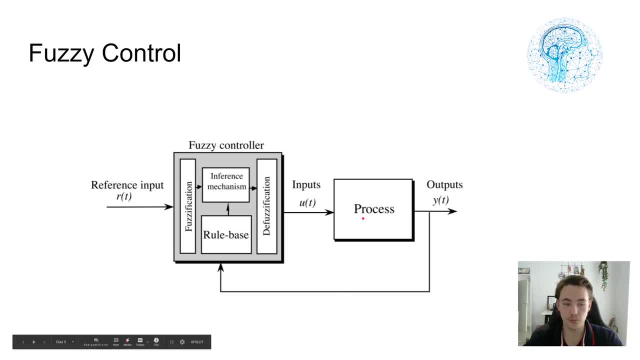 so here we have an overview over like fuzz controller, as in the previous video, where first of all, we have a reference input that we give to our fuzz fuzz controller and then, first of all, we, our reference input is a crisp set, and then we need to uh, do a. 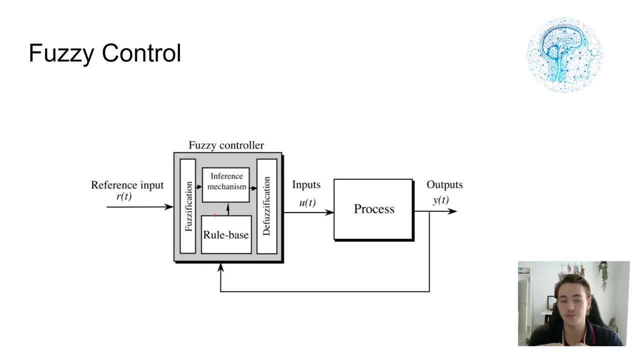 falsification here, where we compare, where we convert it from a crisp set to a fussy fussy set, and then we have like in our inference mechanism here and our rule base that we set up, and then we like inference, um, infer the value that we get into our controller with our rule base, and then when we 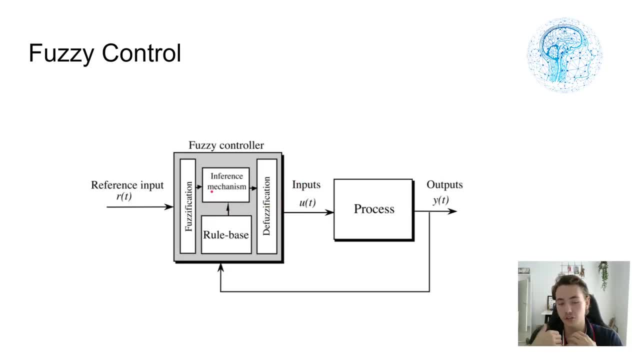 have like um, then we have a value for a fuzz control here. we need to like defuzzicate it, because now we have a fuzzy value, um, and we need to convert that again to a crisp set that we can apply to our process or or in our application or what, what we want to do, and then we use our. 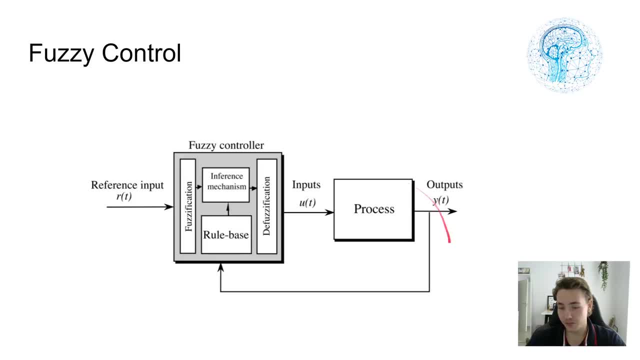 input to the process here, and then we have um, the feedback here from the output to to our fuzz controller again, and this is just like uh, how the, the, the process and like the fuzzy controller works in an overview. and now we're going to talk about like the mechanisms and also like 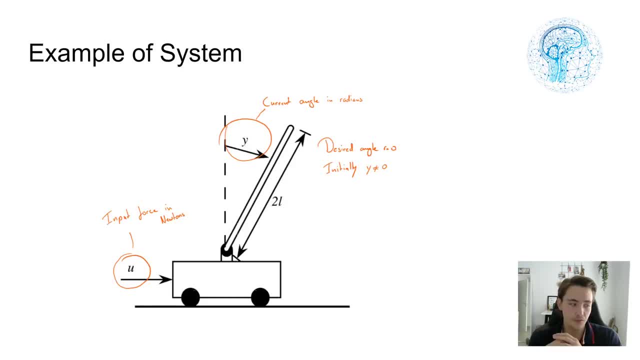 the elements inside of the fuzz controller here. so if you just take another example here of of a system where you have an inverted pendulum that is balancing on a car, so the car here can like with a force here you which the import input force here in Newtons, and then we can push the. 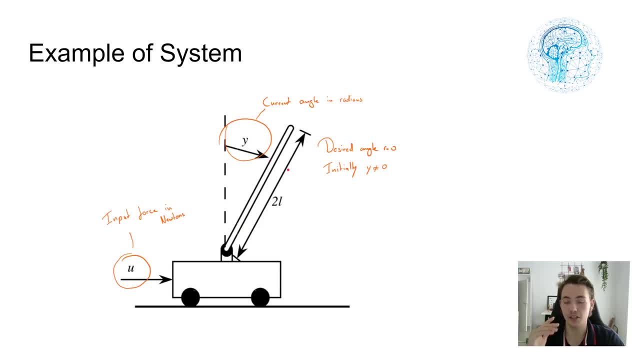 car here, so we're balancing the inverted pendulum here on top of the car and then we have like the stationary position here, which is just like upright here, and then we have like some uh, current angle here in in radians, which is called y in this case, and then it's, it's positive if the, if the. 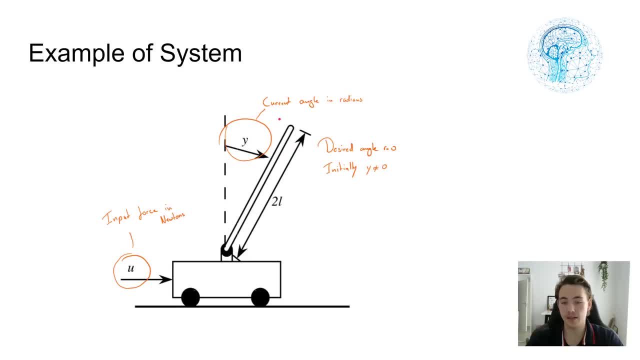 pole here goes to the right. so then we'll get like a change in the angle and like the decided angle is again like equal to zero and initially, like it is initially what we it is, it is not in the server position, so we've been like initialized uh, somewhere from the, from the stationary position. 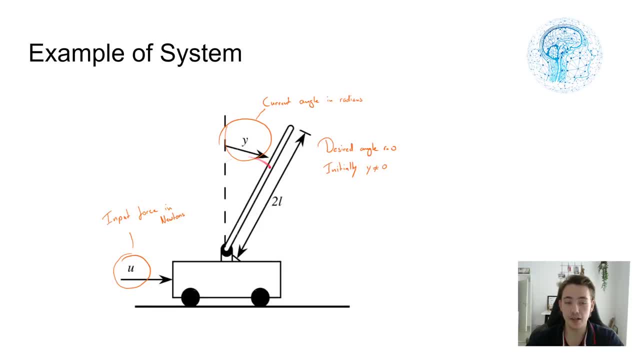 so if we just like have this assembly system here and and our, our pole starts to go like more to the right here, we need to like uh apply some input force here to the to the car so like it will go over here and it will try to like uh get this pole together in an upright position again. 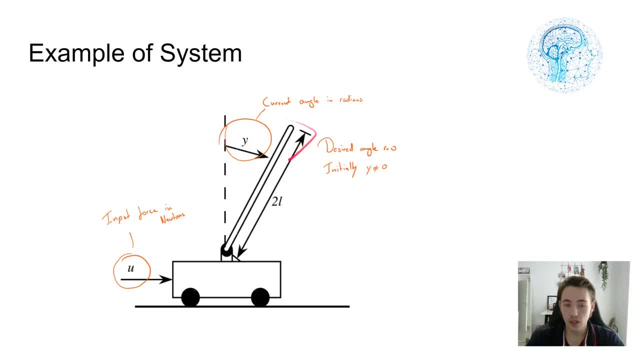 but then we need to know, like we need to set up a fuzzy set here for, like how, how big this angle is here and how much input force we need to uh, to give the system here. so, in case, like our, our pole here goes down here and it's a bigger change in angle, we also need to 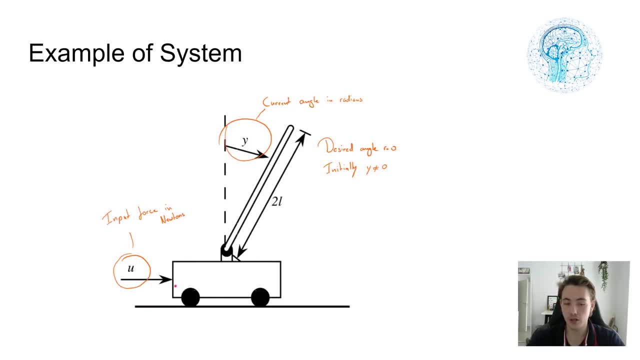 um, apply a bigger uh input force here in Newtons to the car. because if if it's just like a small amount of force here we give to the car, it'll just like keep going down here uh the pole. but if we like push it hard here with a high input force it will go like to the left. 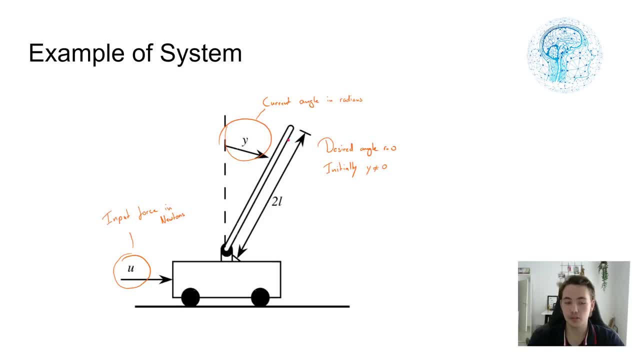 here and we'll try to balance up here. but then if we apply too much um input, input force down here, it will actually like just over swing, so the pole here will just go over here and then we need to like give it a negative force down here or like push from the push from the other side of the 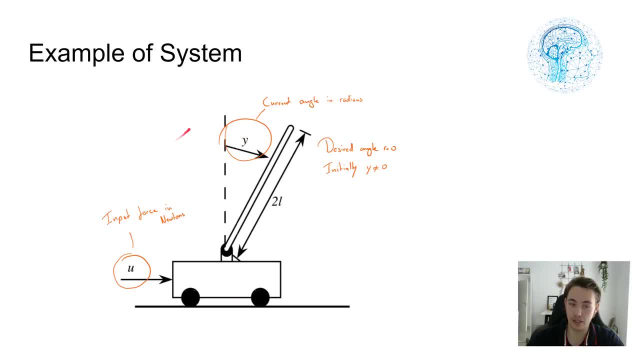 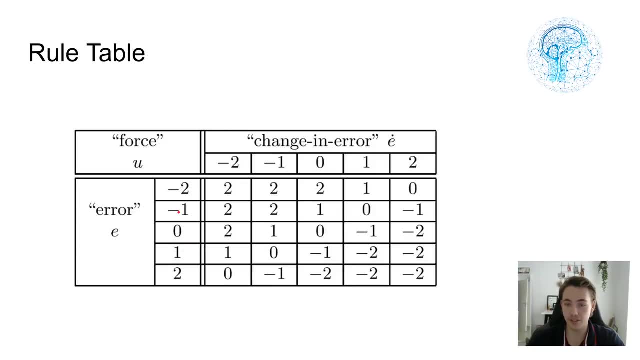 cart pole. so like if, if the angle goes over here and we need to like balance in the other way, so we can set up our rule table for it for uh, for this kind of example here where we have like the error and then we have the derivative of the errors, which is just the, the change in error. 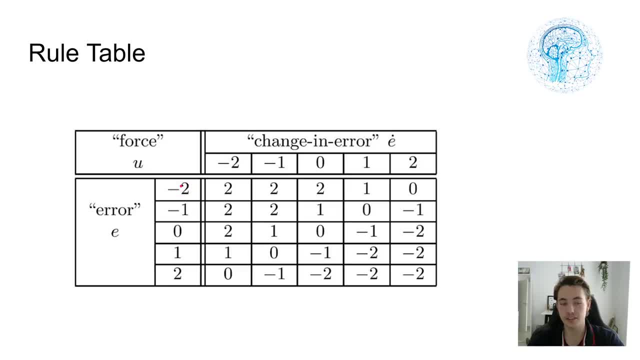 so like if the error here like let's say, um, it's a big negative uh error we have and the change in error is big as well. so our angle is is pretty like it's pretty far away from the stationary point and it's moving uh kind of fast and we need to apply a positive um input force. and if we just 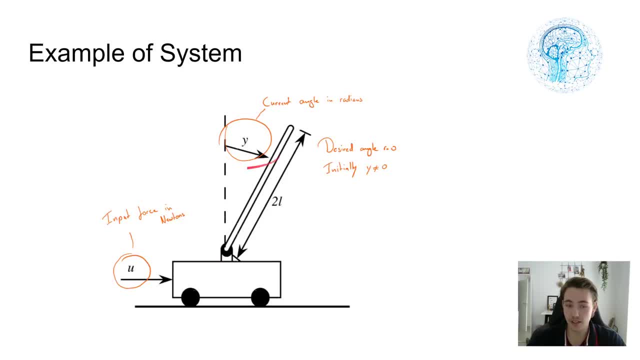 go back here again, we can see that this is the example here where the angle is is big and it's changing, like the angle is changing uh fast. so we need to apply like the biggest force down here to to be able to like balance the inverted pendulum here and then we can just set. 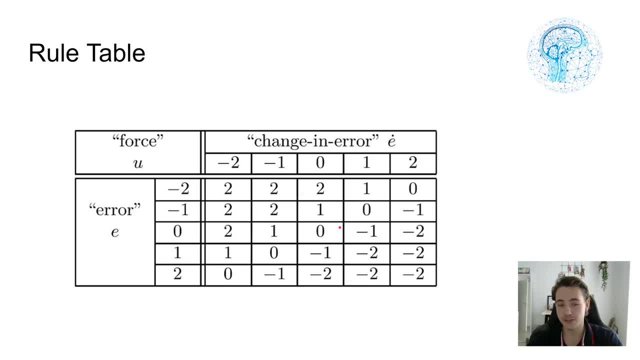 up the rule table for, like all of the different kind of um situations that it could be in. so, like down here, like we have the stationary position here and if the stationary, if it's stationary position, but the change in error, like if we're getting a bigger change, uh change, then we need. 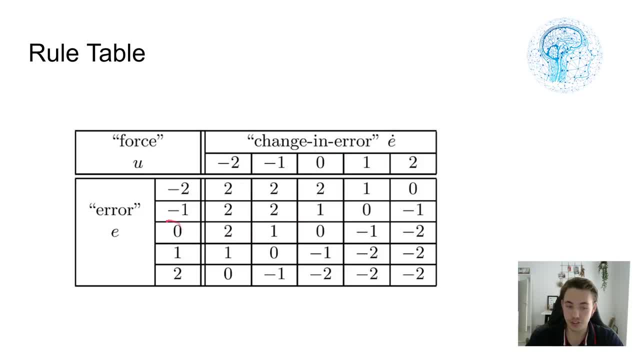 to like apply a bigger force as well. but if we're in stationary position and there's no uh change in the error, like or like it's just still, then we'd apply no force, because then we're just at stationary position. or if it goes like the 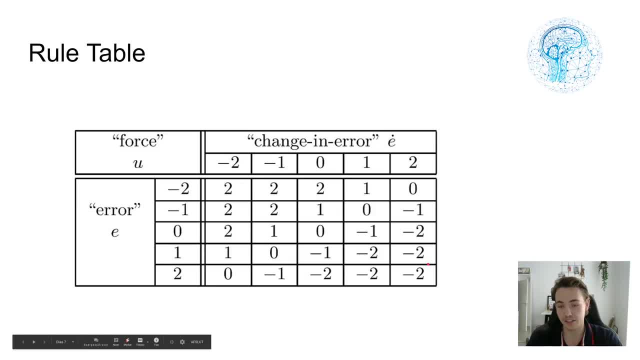 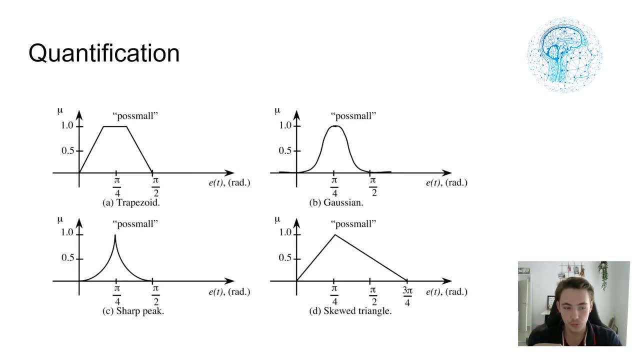 other way- uh, the inverted pendulum- then we apply the negative force down here, so we can set up a rule table here that we can apply inside of us, uh, inside of our fuzzy controller, and then we can use them. we also need to do a quantification when we are, when we're talking about, like um, 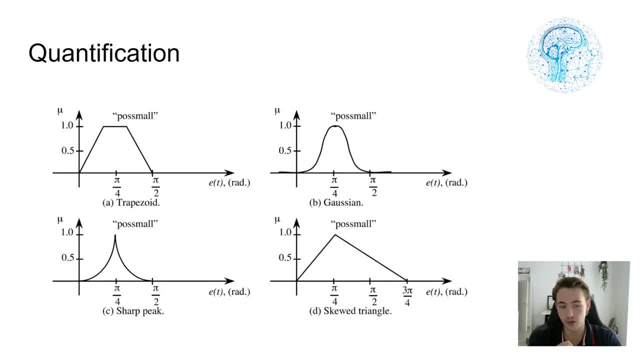 a fuzzy controller where we set up our memory, memory grief, uh ship function, um, and then it can actually be arbitrary, like you can choose whatever uh membership degree of uh membership function uh that you want to. it can be like some kind of uh travisoid um um function, or it can be a. 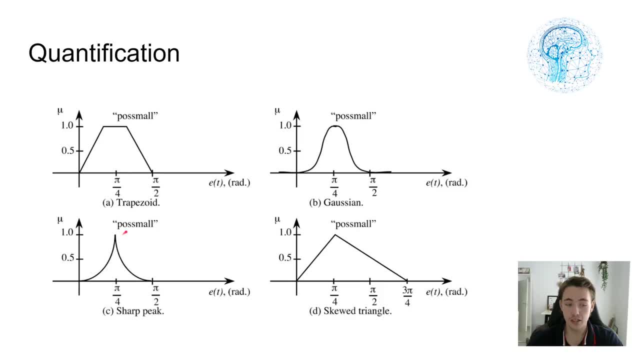 gaussian. um, a sharp peak if you just want to like it is only, like it is only valid for like a short time, like only at a pi divided by four. it is like it is if it is fully true and then then else it just like uh, falls, like it's some kind of like in exponentially, you know. so that's kind of the thing. 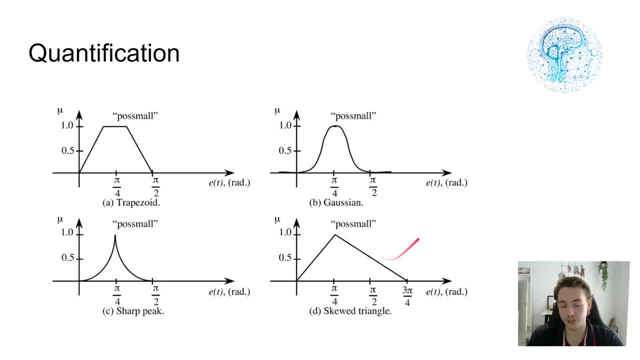 i'll have like screw triangle, or we can have like some kind of waves, if you want to, if you want that and if that like fits until our fuzz is that that we set up so often we just use like the, the triangular, um the triangular function, or like the gaussian function, um up here. 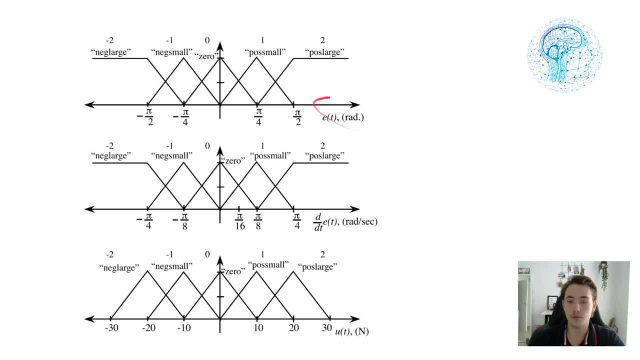 so an example: we just went over here, we had this error here and we have like the change in error and these are two inputs to our uh, to our controller, and then we can set up this um membership degree function, um inside of like our, our um, our coordinate system here, where we have 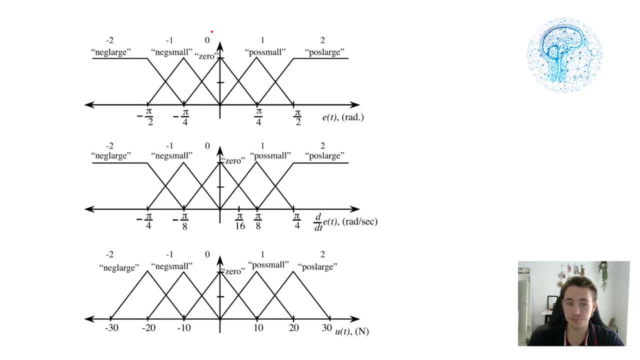 like our universal discourse out here on the x-axis and the membership up here on the on the y-axis. so we can see we divide our, we divide that fuzz set into like neck large and next small. so it's, it's the, it's the angles. um, here it's the, it's the, it's the error in the angle. so here, like we're, 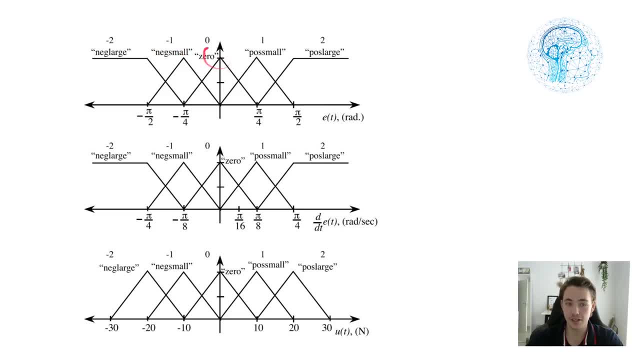 the pendulum is to the left, like it's it's a little to left, and here it's stationary, and here it's it's a lot to the, to the left and over here to the right, of course, and then we have the radians down here, um, as as the error, um, and then for our zero, here is the stationary position. so if we would be, 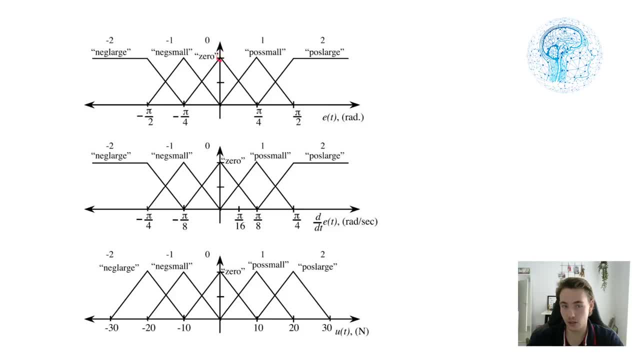 in the stationary position, our membership degree of um would be uh one, here with the, with the rule here zero. so we also have to like the same down here and we just use the triangular membership degree function here, in this case um, and down here we have the change in error, which is also an input. 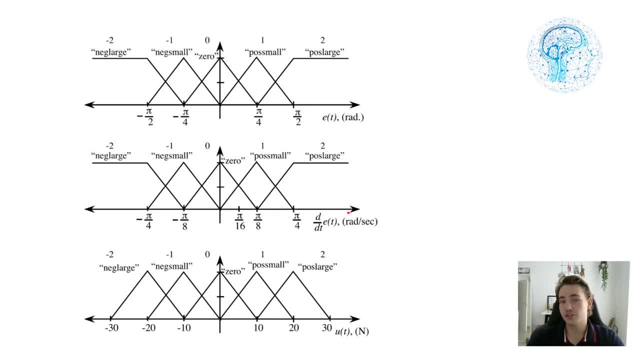 system and which is just radians per second. so it's it's how fast our angle is changing and it is just like um, the same as the rule set that we just set up, but we use a triangular membership degree function down here in in the button here, where you can also see like it goes to like um. 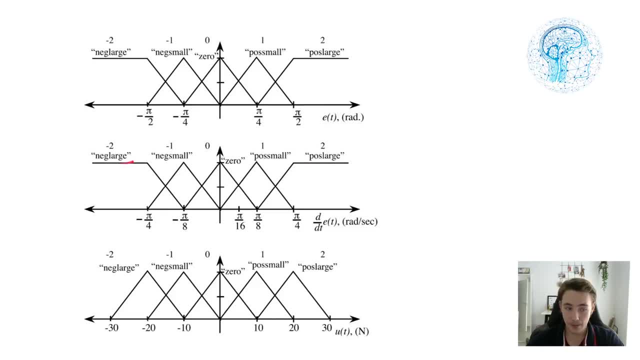 minus infinity here and positive infinity here. because if our, if like our angle it just keeps going down, it just like it just goes out to the left and and we're just neck large because we can't see it. and the same if it goes to the right and just keeps going down to the right. 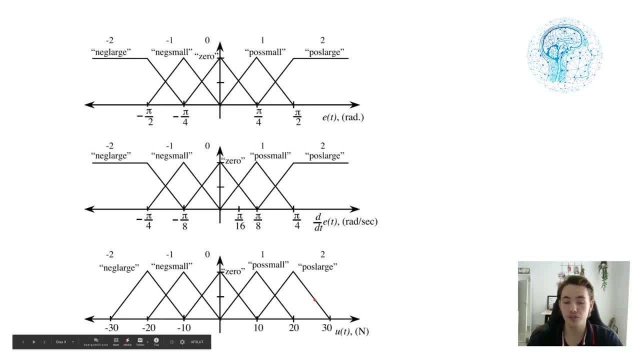 so down here in the last year, we have our, our output from the uh, from our fuzz controller which can, which is like the force here that we need to apply to the card um, and then we also like, just set it up in our fuzzy set here with neck large, next small, zero possible and plus large with 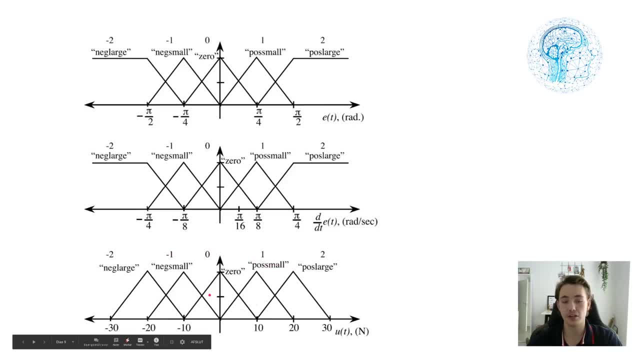 it with the, with the, with the triangle of membership degree function here again, and then we just apply those forces when we're in the control area and then we just set it up in our fuzz set here in different kind of situation up here, as we just set up it now in our rule base. so this is just 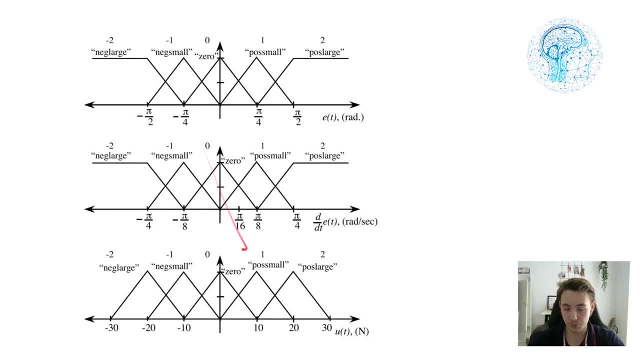 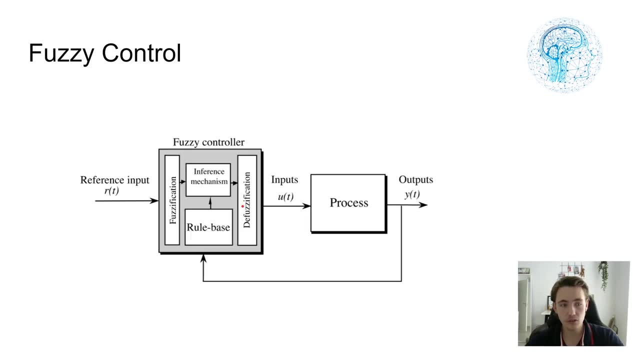 like a visualization with the, with the triangular um membership degree function, um, of our rule base that we just set up here on the previous slide. so again here we can just set up our fuzz controller. we have now talked about like falsification and our rule base and inference mechanism. 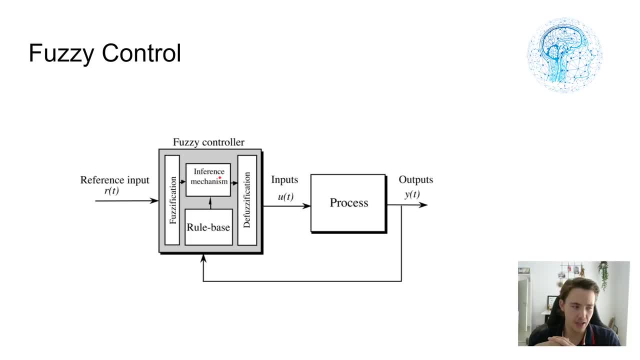 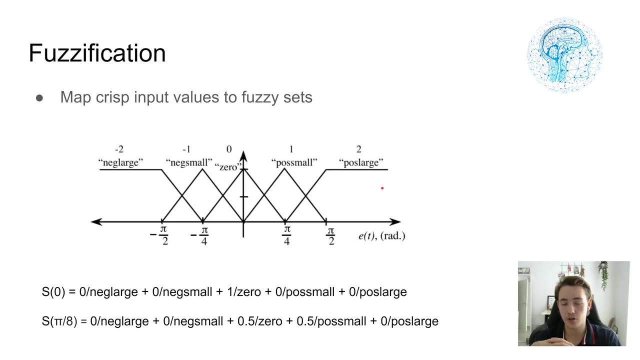 but then in the end we need to, when we have made our choice and we have get uh, get a, when we get a fuzzy value, we need to defuzzificate it to get a crisp value that we can actually apply to to our process. and first of all, we need this falsification here where we map, map our crisp. 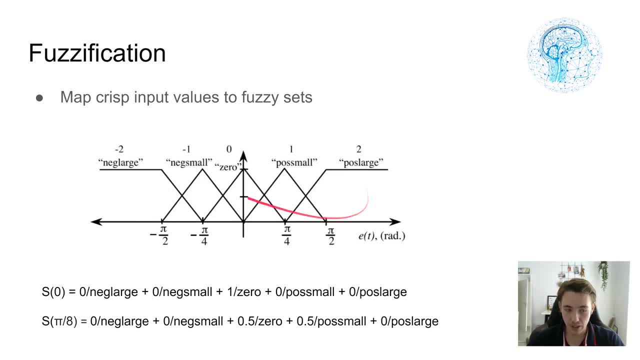 input values to fuzzy sets, where here we have, like some, it can either be like um here in this case, here we have like s of zero. so now, now we're, now, our pole is at the server position, so we have no value here for the neck large and we have zero value here for the uh. for the next role. 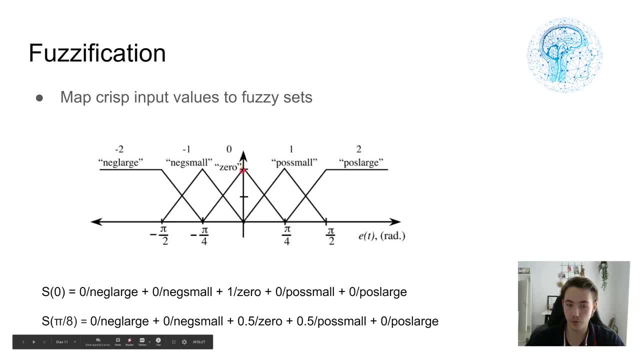 but we have a one here for our zero, because we're at the stationary point, so it will be right, right here and no values for the rest as well. but let's say: here we have like, for example, our s of pi divided by eight, it will be like um here in the middle of like, it will be here. so we have like. 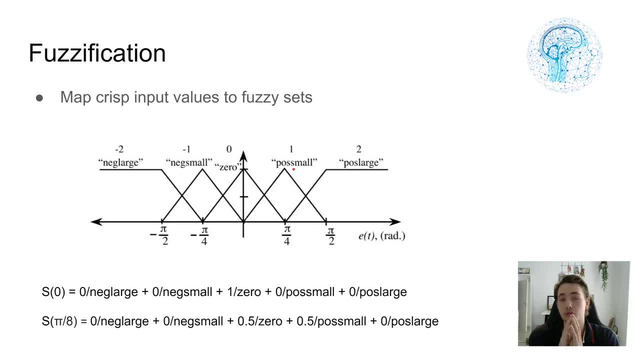 we're in between like zero and pause small. so we're in between like two uh fuzzy sets here. so again, we have no values for neglect, next mold. but we have a half here, we have the 0.5. we have 0.5 for our zero set here and 0.5 for a possible set here. so we're just in between these. 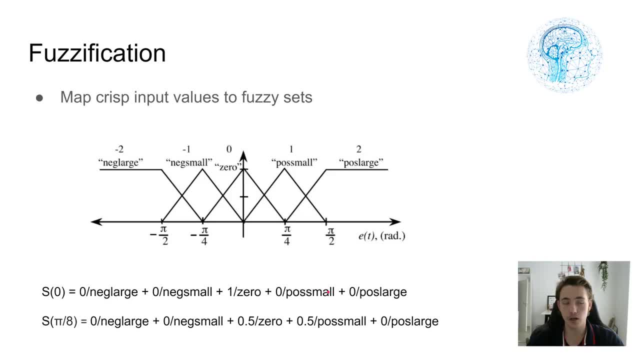 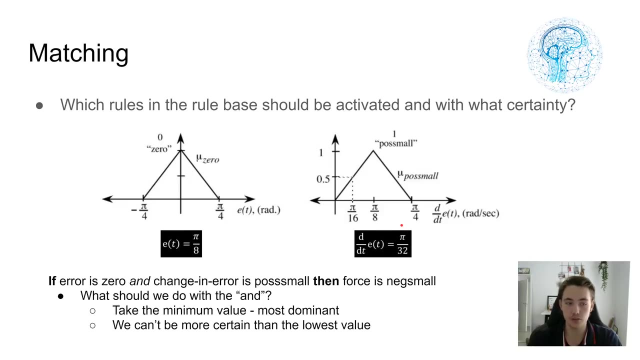 two sets. so this is like how we set up our, our classification and like determine where we are um where we are in our membership degree function. so when we have like our classification we can then match with our rule base, so which rules in the rule base should be activated and with what. 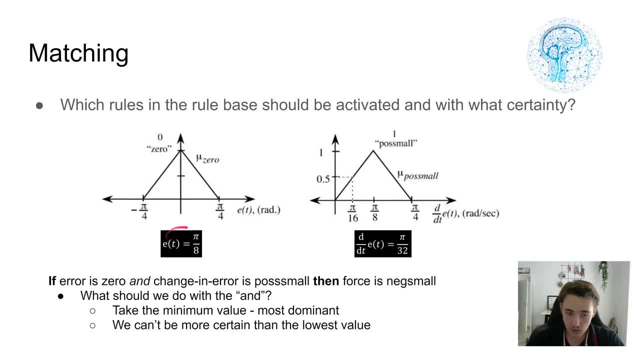 so down here we can, for example, see here: if we had like uh pi divided by eight, we can see like it will be, it will be here. and then we have like this 0.5 that we just talked about. but then, if we like, take the derivative of that error, we can see, like how fast the angle is changing and over here. 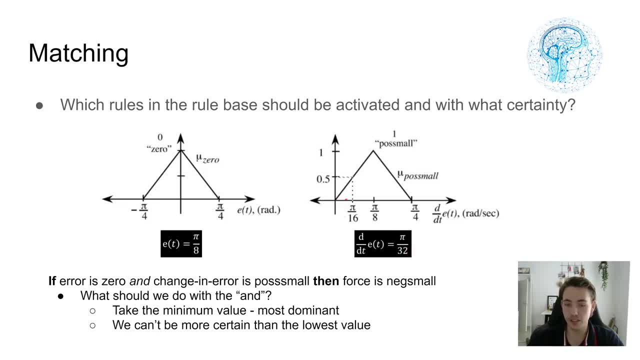 we, we can see, like we have pi divided by 32 and it will be like around here and it will be like 0.25. so now we have two rules, uh, that are activated, but we need to like know, like with what certain t we need to to activate our rule form, and down here just wrote that this is just a condition, that 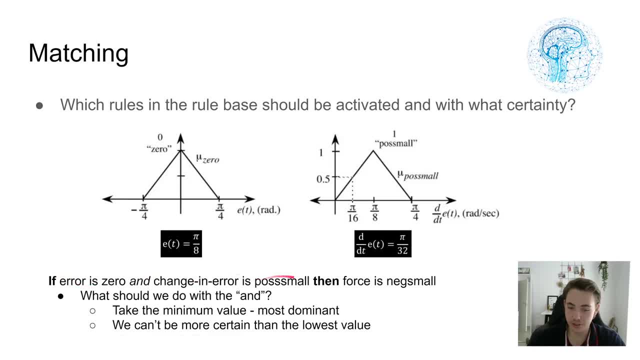 is true now. so if error is zero and change in error is possible, then we need to apply the force next small to our system. so what should we do with the end? because we have two rules that are now activated, so we can either like: take the, take the, take the minimum value, so it will be like the most. 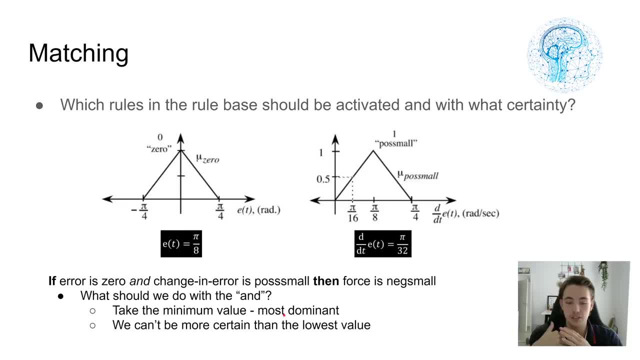 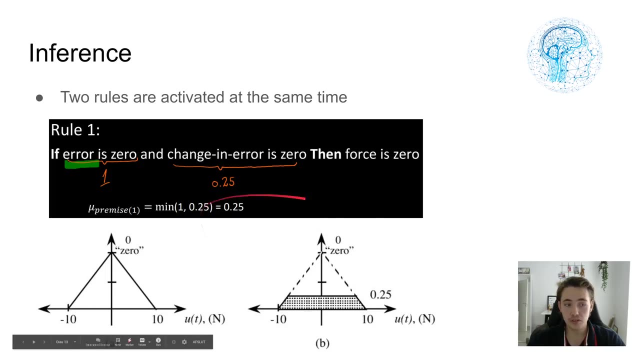 dominant value and like because like the lowest value will also be like the most dominant value. so we can't say that it is like more, more zero than possible, but because like possible is more dominant than than zero and we can like be more certain than the lowest value. so this is just like. 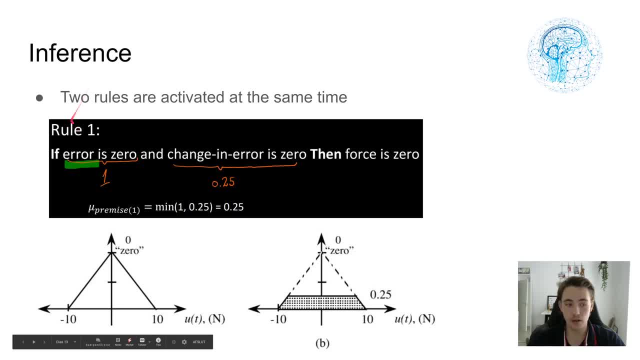 a continuation, for far from from this example here, where we have two rules that are activated at the same time, and the first rule here is that the error is zero, as we just sort it so here that we are at this point here, and then the change in error is 0.25. 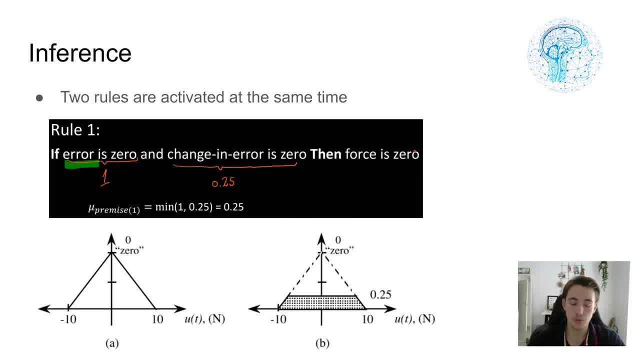 five uh, then we then this, then the force is zero. but we need to like, know, like what, what certainty we need to apply to our uh activation. so we just take the minimum value of d2, because we are operating with the end here, so we have two rules that are activated at the same time, so we just 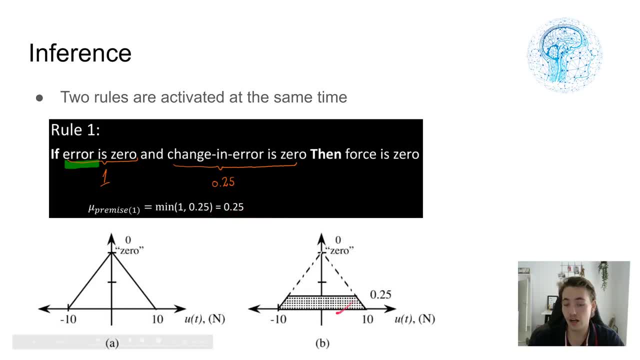 take the least value here, which is 0.25, and then we do our alpha cut down here, so our our membership degree here in this case, for for this rule that is activated is the area down here, um, in the triangle that we just cut out with our alpha cut here at 0.25. we can also have, like the 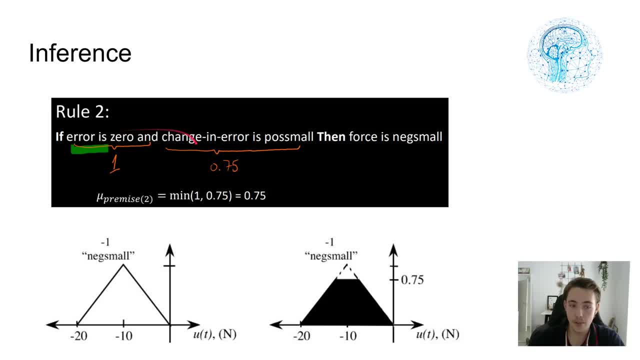 second rule: here that is true, and it is like the error is zero and the change in error is possible. so for our next small here we have like 0.75, and then the force needs to better, need to be applied is the negative small input force, and then we take the minimal value which is indeed like 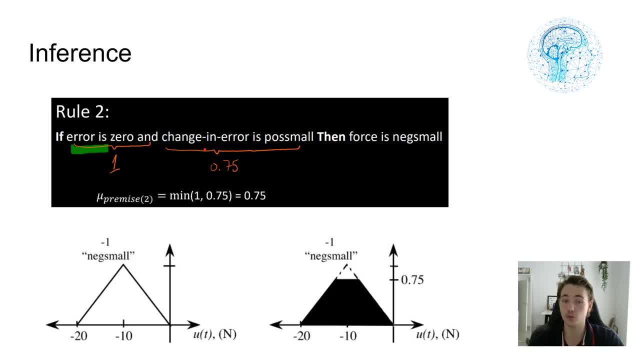 0.75, because we're using this and operator here's, two rules are activated at the same time. then we do our alpha, cut here again um 0.75 and we get the area down here under and then we have: when we have these two rules here, um, and we have these two rules here, we can like put them together. 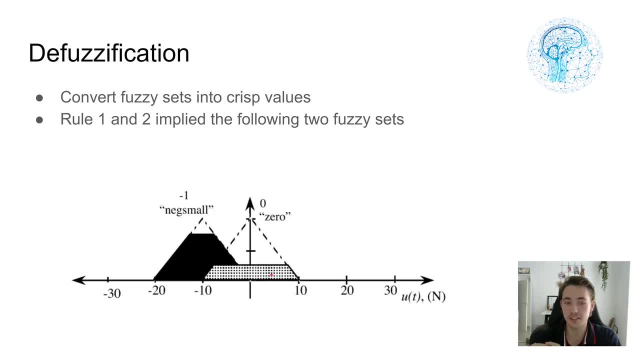 and when we do deflasification, we need to convert our fuzz sets into crisp values. so these are these, like these, uh, like um, these great, our areas, or like dotted, like dotted areas here, like they are the membership degree that is applied in in this situation, right, 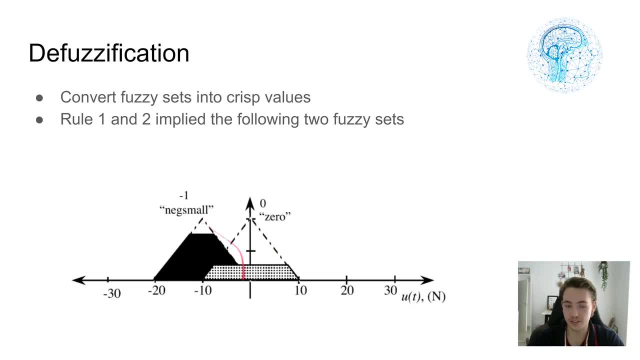 now and we'll want to imply the following two fuzz sets. so, as i just said, it's just like the areas down under here in the triangle that is the case now and it's our falsification um that we need to like defuzzificate to get a crisp values for these values again, and there are different kind. 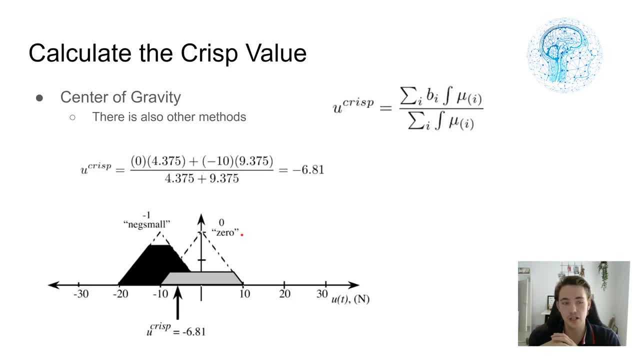 of methods where we can calculate crisp values from um. one of the examples that uh, or methods that we can use, is to use the center of gravity, and there's also, like, a lot of other methods that we can use. so in this case we're just using, uh, this end of gravity, which is like the point. 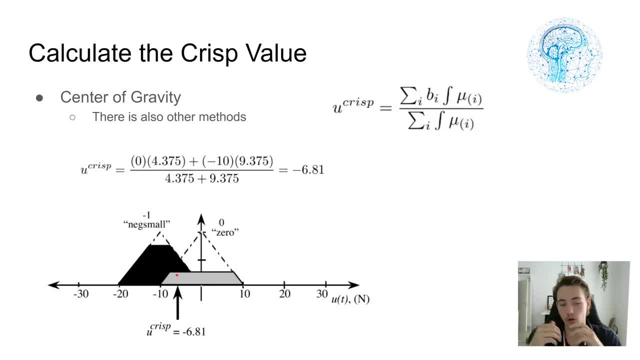 where like, where like um, this, where like it's, it's all like in the middle, so it's like the center of gravity. yeah, and then if we just plug it into this formula up here to calculate the center of gravity, we get a value here of a minus 6.81, and this value here will be our. 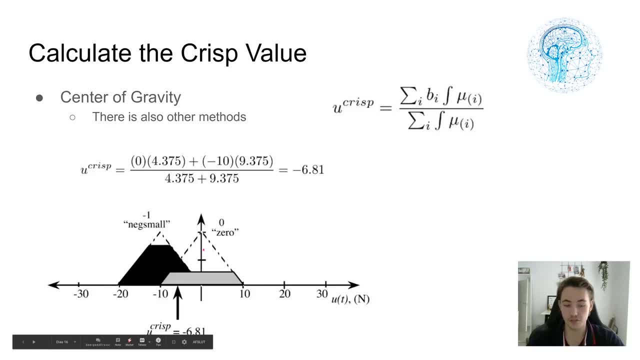 our crisp value for our falsification, or from our fuzz controller. and in this case, here we can see that we need to apply a negative force on our card, um, like 6.81 and newton to our card to like balance this. um, this car like this. 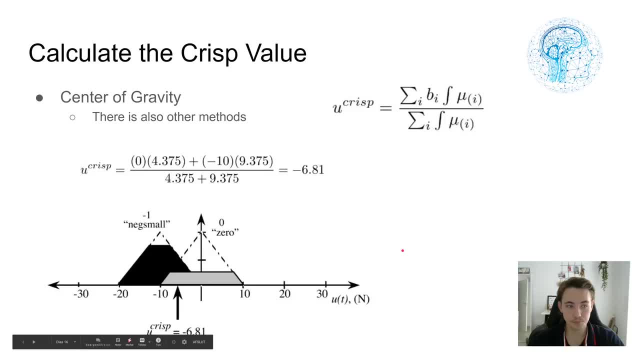 pole, in this case, here for um, for our thoughts. so that's it for this video, guys, and this we have been. we have been over like the fuzzy controller and each element in the fuzzy controller, how we can go from a crisp, crisp value and do some different kind of stuff in our fuzzy controller. 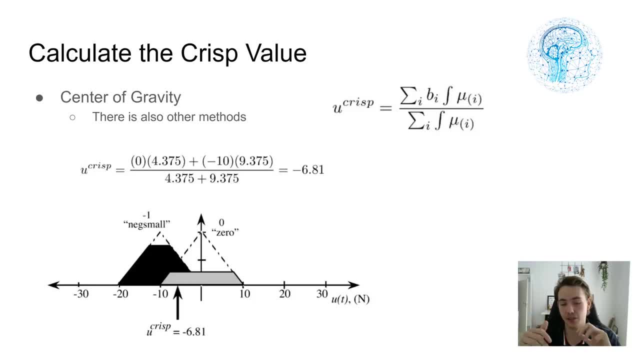 with our rule base that we set up and then get a crisp output again that we can apply to our system. so in this case here we just in all the time trying getting an angle and changing angle to our first controller and then every time that changes like we get a new. 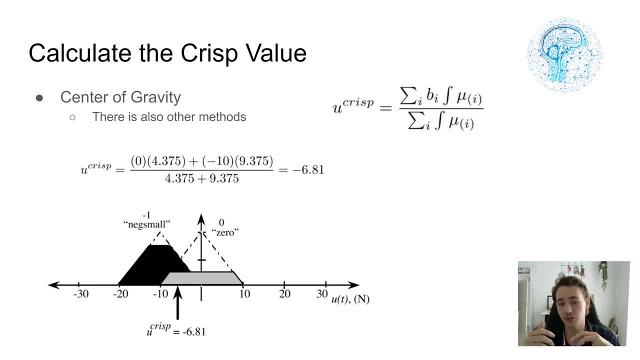 value for our crisp output, which is the newton that we need to apply to our car. so we're always trying to like balance the inverted pendulum from some given state um on top of our car here by applying some force. so this is like how we can like the different kind of steps that that is needed. 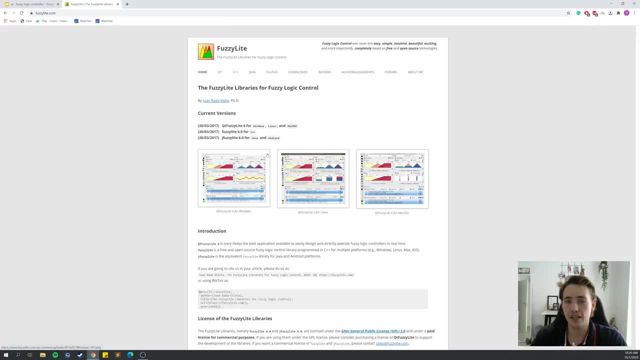 and then in the next video here i just want to show you like that we're going to like implement a fuzzy controller and ourself where we use this as a library or api- here that is called fuzzy light in cyprus plus- so we can actually like go into c++ and set up our 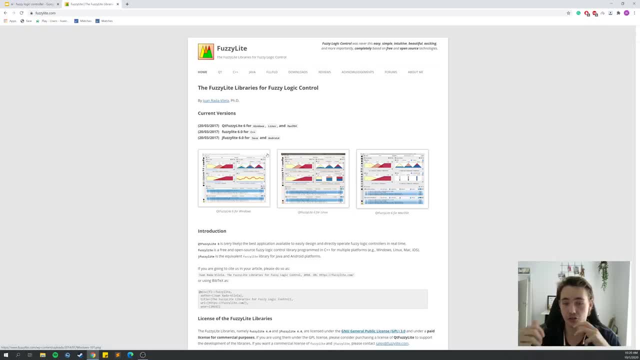 rule base and do different kind of stuff, um with our first controller and also, like, define our membership degree function and our set, and then we can actually implement a fuzzy controller which we can give an input, and then we get a crisp output that we can apply to india. 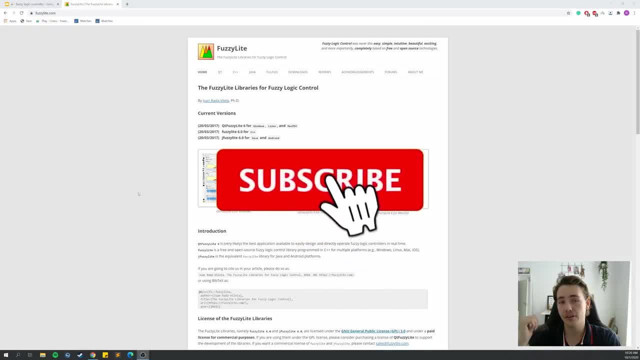 system. so thank you, guys for watching this video and remember to hit the subscribe button and bell notification on the video and also like this. like this video to show the youtube algorithm that you like this content and you want more of it in the future. i'm currently also doing this algorithm. 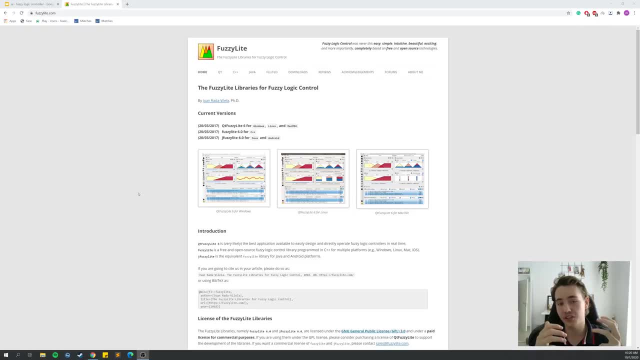 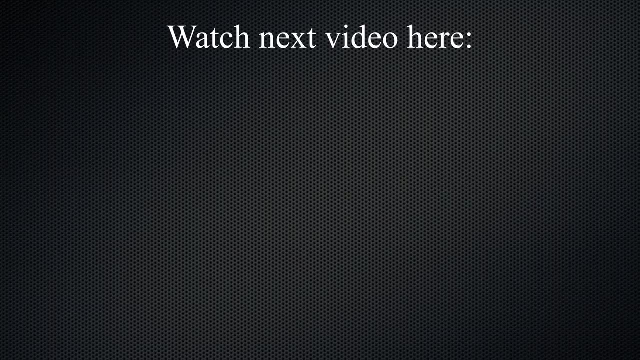 data structure tutorial in c++ or the computer vision tutorial with opencv. so if you're interested in one of those, i'll link to one of them up here, or else i'll just see in the next video. guys, bye for now you. 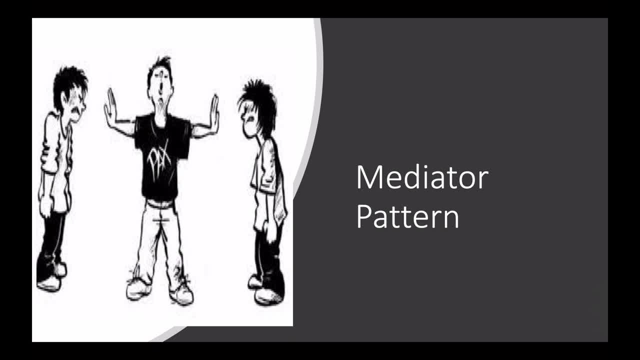 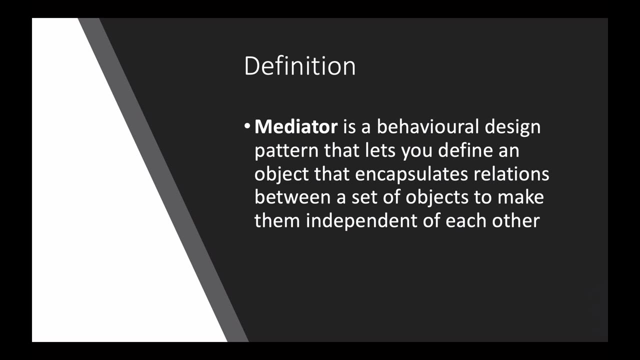 Hey everyone, this is Chiranjeevi, and in today's video we are going to talk about the mediator design pattern. So let's start by taking a look at the definition. So the mediator design pattern is a behavioral design pattern that lets you define an object that encapsulates relations between a set of 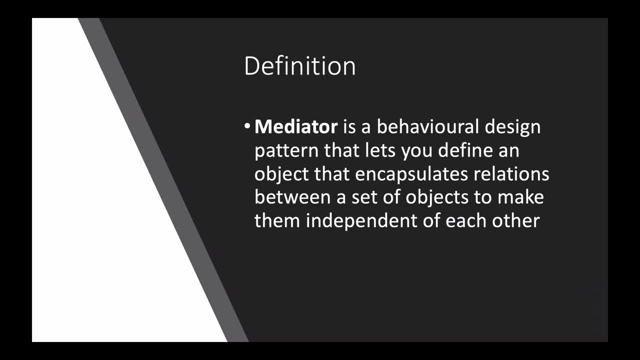 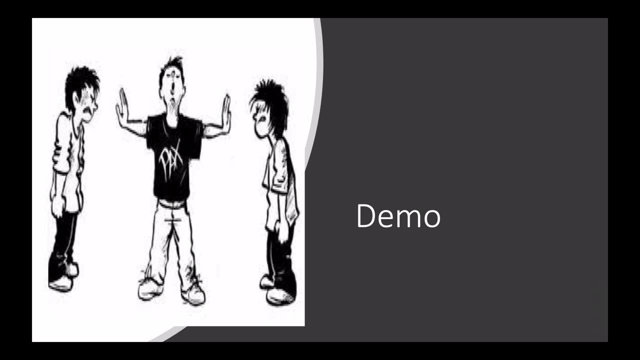 objects to make them independent of each other. So now the best way to visualize the mediator pattern is to look at this diagram. So now you see that there is a guy standing between these two guys and they are about to like, do some fighting or communicating or whatever is it, but this guy is like: okay, whatever you want.